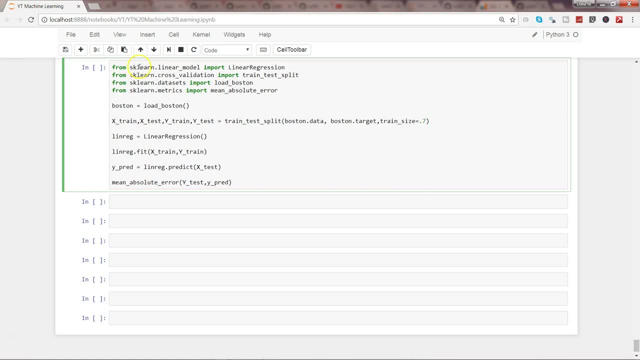 you in previous videos that first of all we have gone ahead and imported the linear regression from sklearnlinear model, then we have gone ahead and imported the train test split from sklearncross validation and then from sklearndatasets. we have loaded the boston data set to predict the house prices and from the sklearnmetrics we have gone and 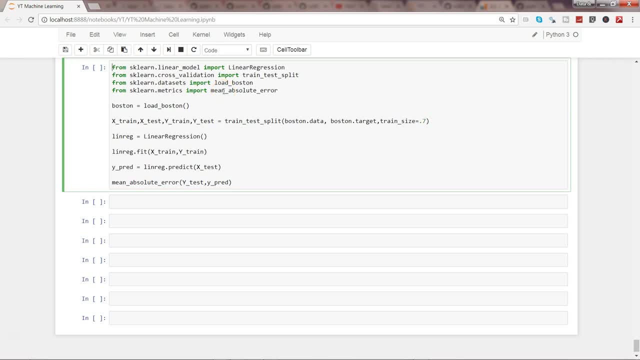 picked up the mean absolute error as to test how well our prediction is doing when we compare with the test data. so now we are going ahead and loading the data. after you have loaded the data set you, we need to use the train test split to split the data. so what we are using? 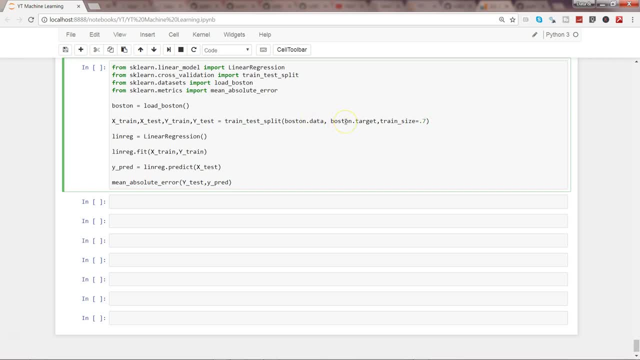 is bostondata, which is all the x variable, and bostontarget, which is all the y variables, and then the train size is. basically we are saying that 70 percent data should be used on the training and rest of the 30 percent on testing. after that we are initializing the linear regression. 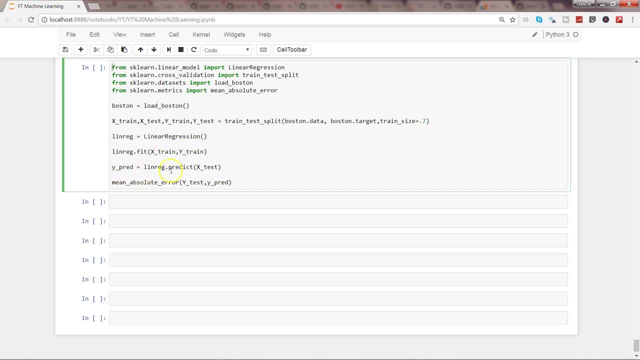 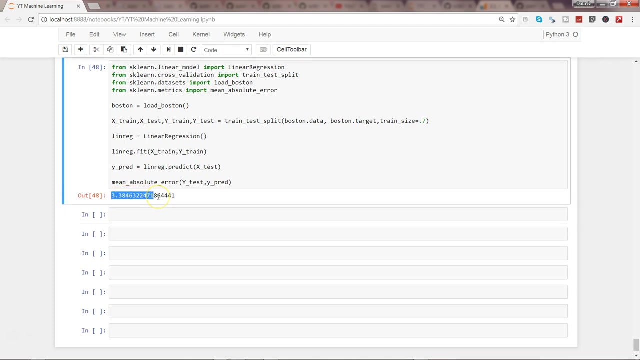 fitting the linear regression with the x train and y train data, predicting it with the help of the x data and then identifying the accuracy with the help of the metric mean absolute error. so let's go ahead and execute this. so once we execute this, you can see that mean absolute error is 3.38. now the 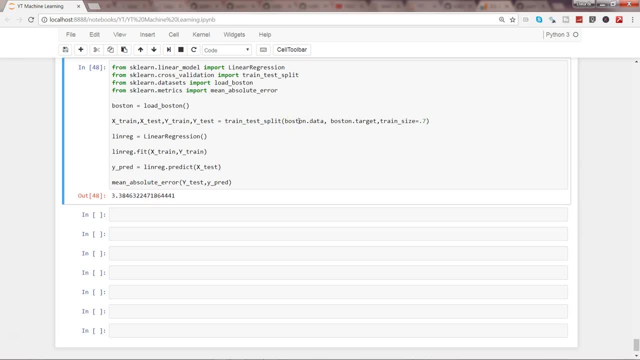 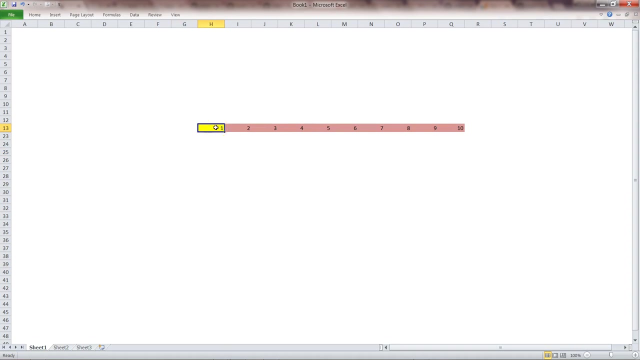 issue is that you are only looking at one set of data. so what you have what? what i mean by that is data- is interest training and the rest of the 30 percent is testing. so if i visualize this, you can better understand. so if i go to my excel sheet, so what i have here is basically the same representation. 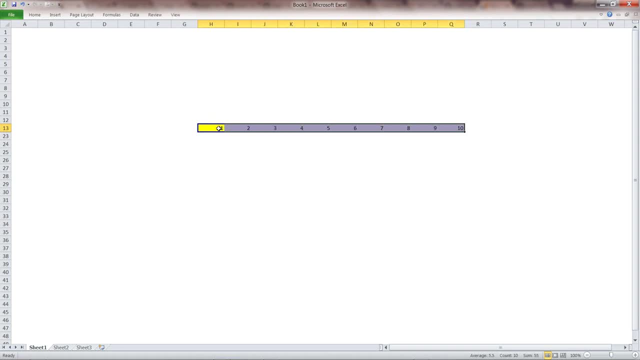 if you can ignore these numbers for a moment, what i'll do is i will just make it white or maybe delete it for a moment. so what i mean by this is this: this particular section is basically- you can think of 70 percent of your data used in training. 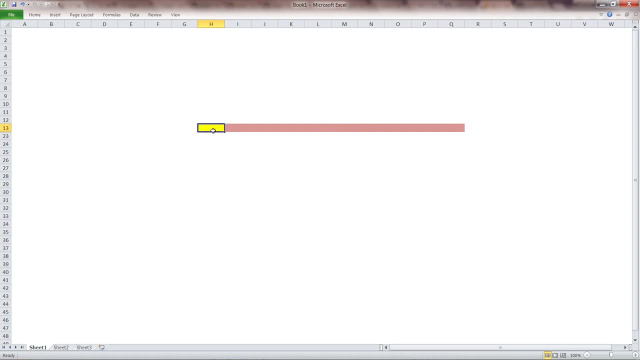 and this 30 is basically the testing, so that's like just one picture of the data. wouldn't it be nice if this 30 is like shifting here, then here and then here a couple of times, based on you specify that i want to shift it like 10 percent, so that you are basically iterating all of the data. 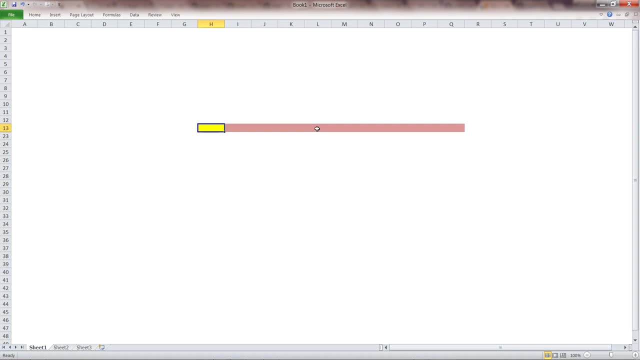 by splitting it into training and testing and then creating the average accuracy. how it helps us is basically when you are doing the training and testing split strategy with this map, with this way, where you are changing the test site anywhere between the training data by taking that portion. 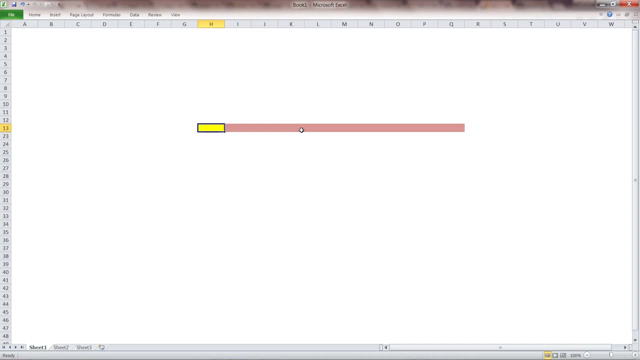 then you are basically moving around on the entire data set and you can get a different accuracy scores and once you average it you get an idea about the entire data, that what an overall accuracy score is, and this will then further help that if you are, let's say, want to predict with the 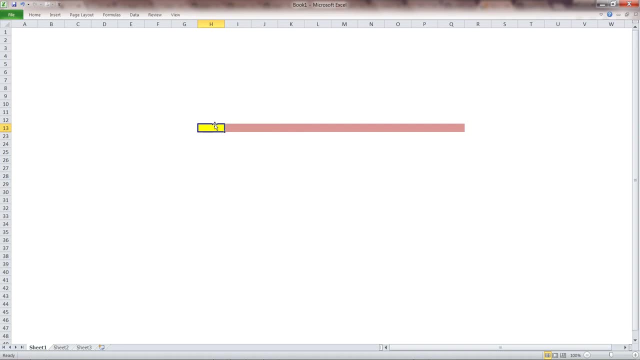 linear regression or with some other type of regression like the random forest regression or any other regression method, then you can get your accuracy scores here a little bit faster. so if you have done some really good research in the fields for inter-trans, mycket conoc Yea. weitere информ т россет. 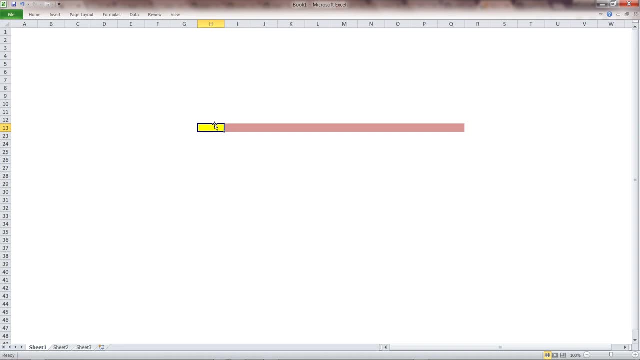 can compare these methodologies as well as for hyper parameter tuning, where you identify whether adding or removing a particular parameter really helps these accuracy scores when you iterate it on, the entire data really helps you and gives you a more finer control on your model. so if I just go ahead and press, 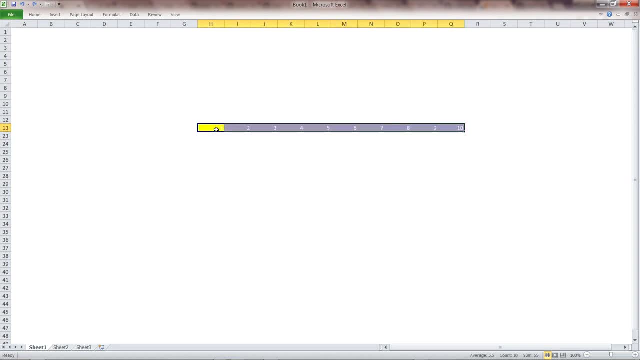 ctrl Z. so what I am showing away, showing over here, is is that we are. I just change the color to black. okay, so what we are changing, what we are saying over here, is that let's divide the data set into in a way where you have the 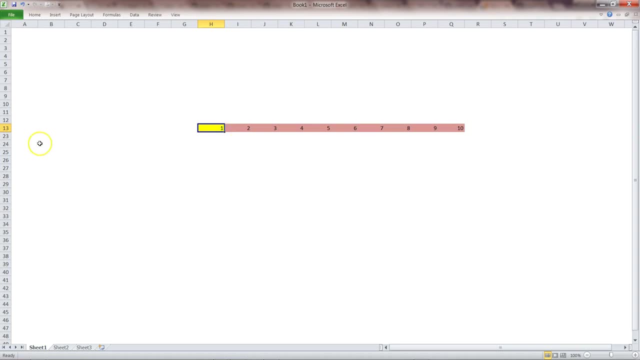 testing 10 times in our data set, so this is the one. so if I unhide this and then, as you can see, the testing is shifting over here, then here, then here, so that way the data set, the testing, has iterated multiple times on the entire. 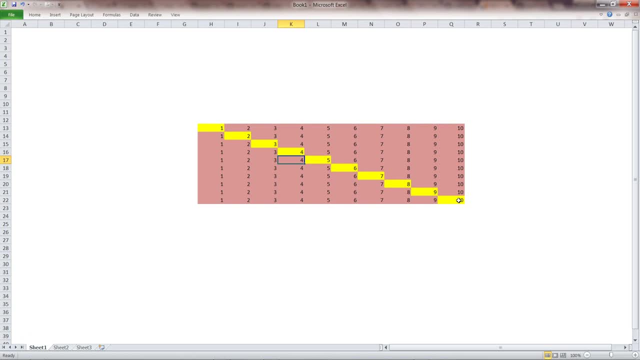 data set and once you average it, it gives you a much better control, and that's what I meant by that. so that's, that's a representation, the pictorial representation, and this is achieved by using the cross validation into the or a cross validation score into the Python scikit-learn. so let's go ahead. 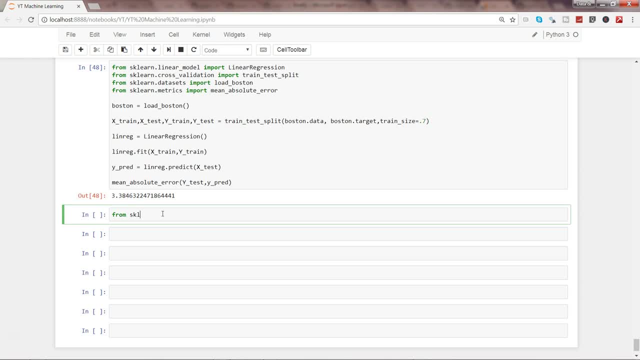 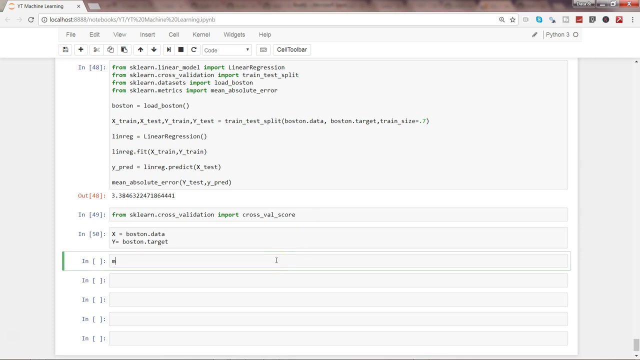 and execute that. so from sklearn, what cross validation import, cross well score. that's what you need to import. and then next take x into ah boston dot data and y into boston dot target. after that let's create the multiple regression by initializing the linear regression and then saying: multirag dot fit x, comma y. 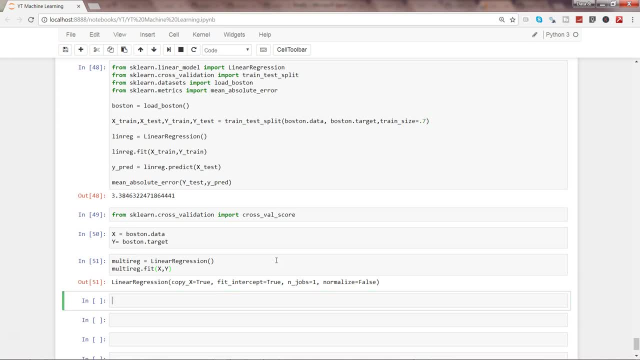 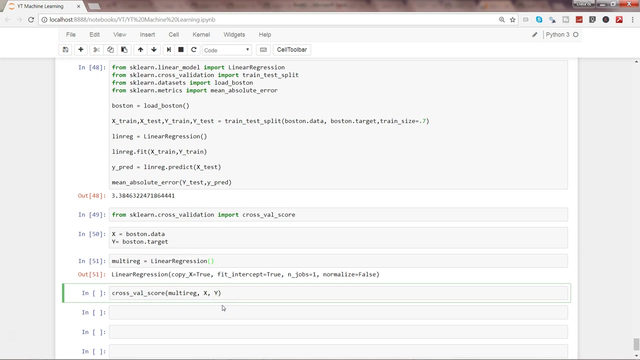 execute that and then, yes, use the cross validation score on the multirag comma x, comma y. so this, this particular section or this particular one, was really not necessary, because that's what we are doing it over here. so multirag x, comma y, comma c, v, which is a cross validation. so how many? 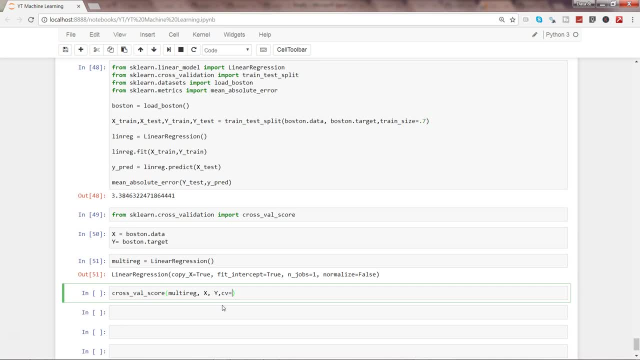 number of times you want to do the cross validation now. it may be five, it may be ten, it may be even twenty. so it really depends on what number you specify. but you should be really careful because if you are increasing the number, that means it will take more and more time to 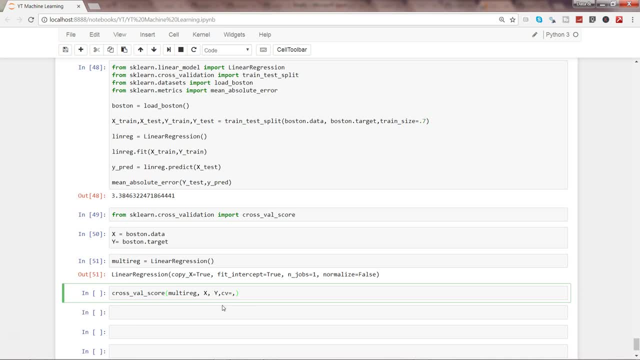 iterate over the entire data, and if your data set is large, it will consume all of your resources and your overall time will be increased. so let's go ahead and start with you five. so what i'll do is i will just, let's say, go ahead and execute that. okay, so here is our 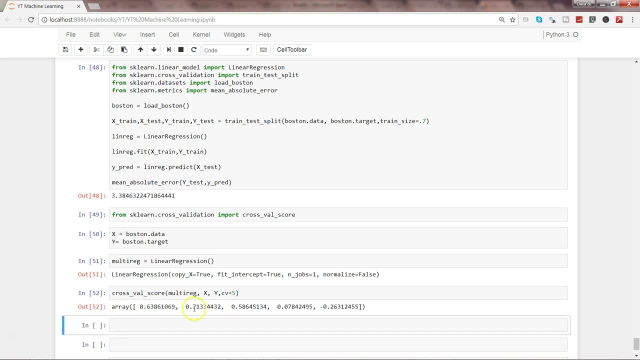 default accuracy scores: 0.63, 0.71, 0.58, 0.07, the negative one. so what i can do is i can simply say: mean, and this will give us overall average accuracy of 0.35. now, if i want, i can also. 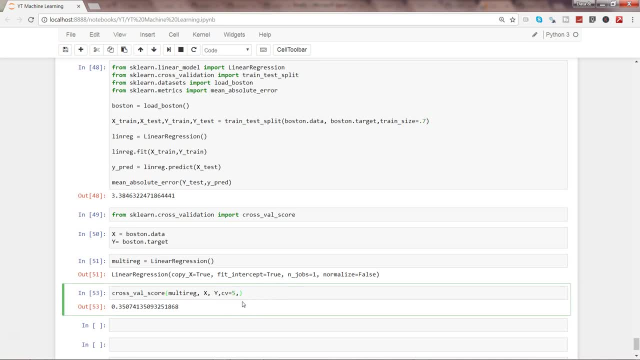 use the accuracy of my type. so what i mean is there is a parameter called scoring and in scoring you can specify what you want. so i want mean absolute error and for that the parameter is: and he underscore mean absolute underscore error if i go ahead and execute, and the problem with this is that 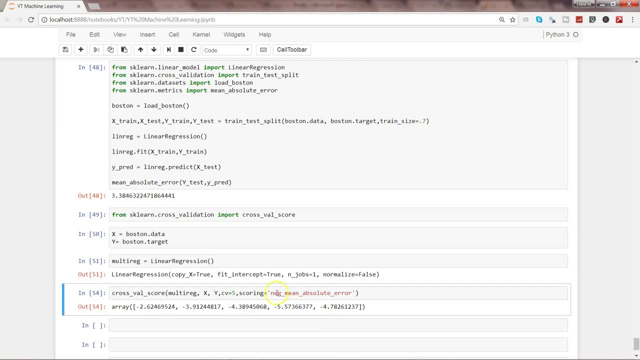 you get the negative scores. and that's what i'm going to do is i'm going to go ahead and execute it, looking for it, and i can see that the absolute error is equal to 0.. constantly, and if you go ahead and execute it, in fact, Professor, you can calcul undermining that we not expect with the mean absolute. 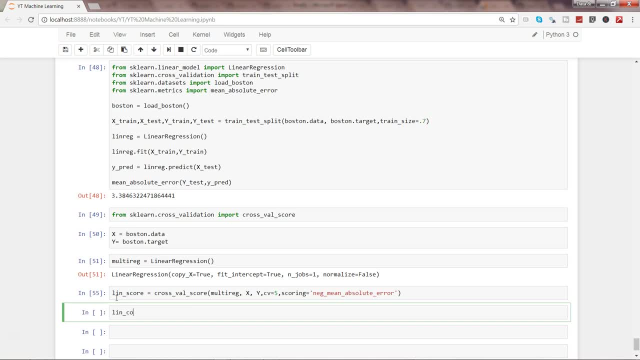 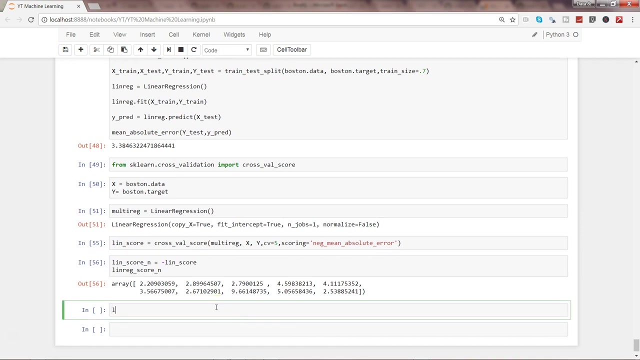 error, because when you do the absolute of a value, it gives you the positive values. what we can do is- and there's an issue with this just doing- is we are changing here and I will simply go ahead, and so these are my scores for linear regression, and if I just simply go ahead and so that's not, 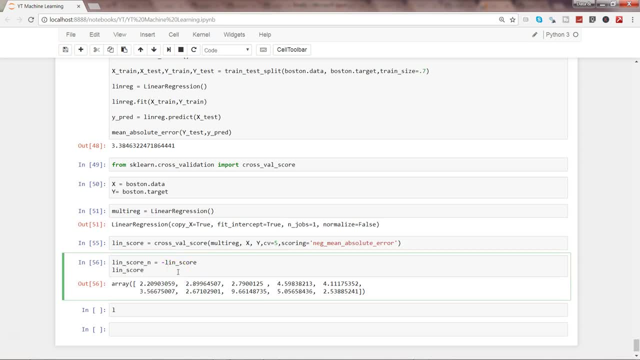 the one and I am underscore, score, underscore and five. I would expect five scores. here are my scores and if I want, I can now mean it and I am underscore score and and we need to use NP dot mean because we are using the mean from the numpy library. and that's basically my four. point two: five based on looking at. 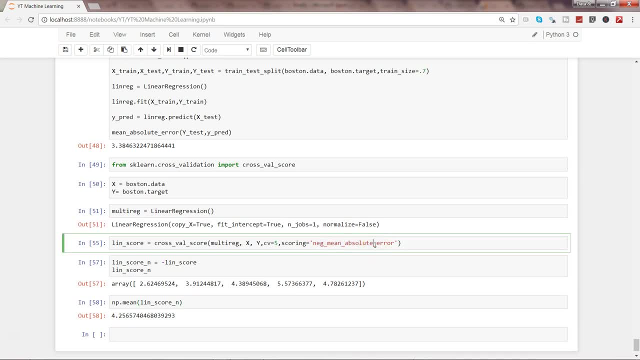 my, my specific error type so you can look at the documentation for different types of accuracy scores that it has. but the idea is that you can use the cross validation to basically shift the testing data at the multiple parts of your data set. this way, testing is happening on the entire data set and the